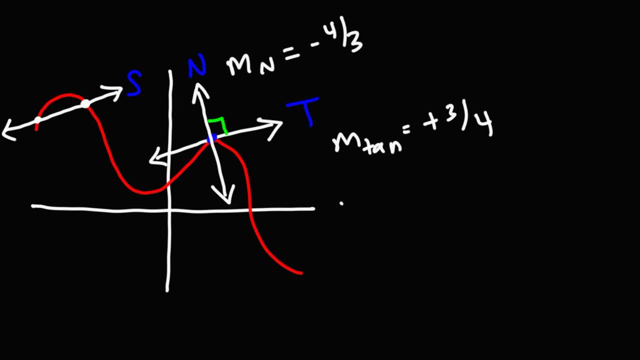 Now the way in which you would calculate the slope of the tangent line. you could find it by evaluating the first derivative at whatever point this is. So let's say, if that point has an x-value of a, it will be the evaluation of the derivative at point a. 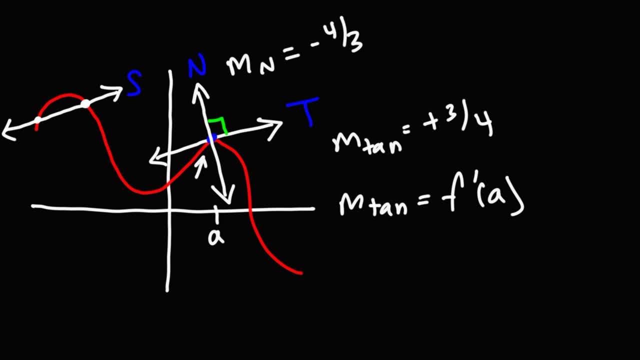 That will give you the slope of the tangent line, which is the instantaneous rate of change of that curve. at that point, Once you have the slope of the tangent line, you can easily find the slope of the normal line. Flip the fraction and change the sign. 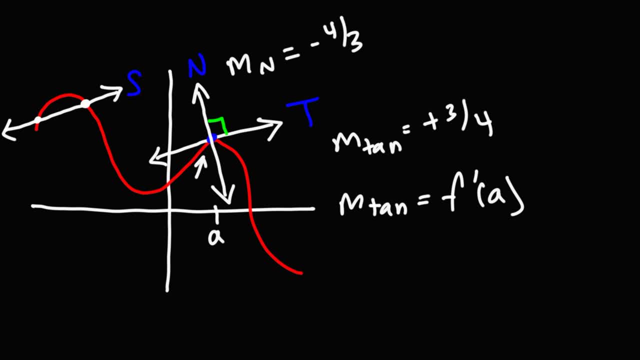 Now, if you want to calculate the slope of the secant line- you've done this in algebra- All you need is the two points x1,, y1, and x2, and y2. And you can calculate it. So the slope of the secant line is going to be: 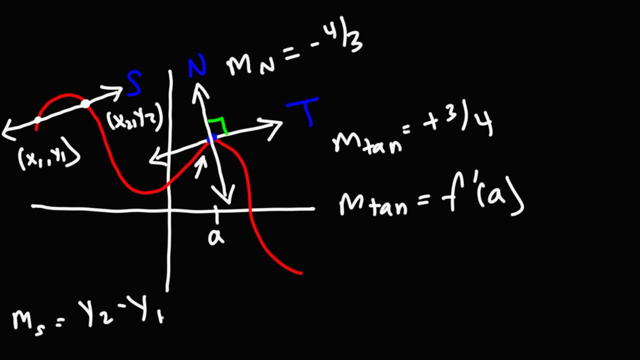 the change in y, which is y2 minus y1, divided by the change in x, x2 minus x1.. Now the slope of the tangent line can be approximated by the slope of the secant line as the limit of the change in y. 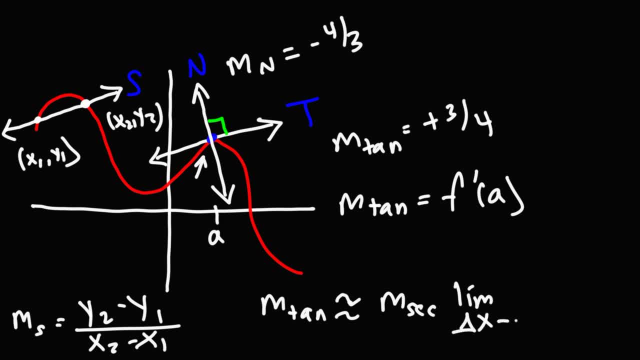 and the limit of the change in x goes to 0. In other words, let's say, if we want to find the slope of the tangent line here, the instantaneous rate of change, at that point we could use the slope of the secant line to approximate it. 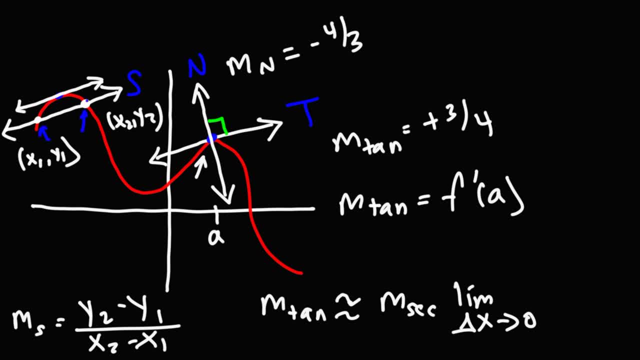 if these two points get closer and closer to this point. So those two points, let's say, if we were to move them here where they're very close to the point in the middle, the slope of that secant line is going to be a better approximation. 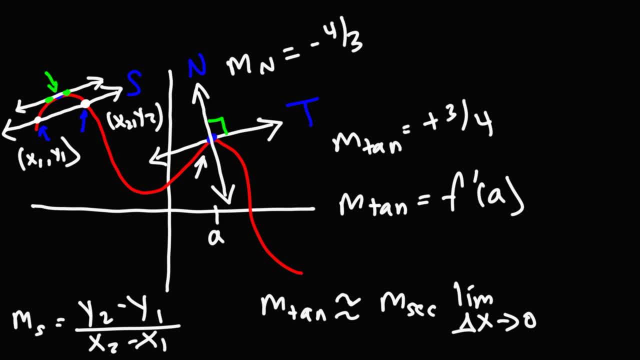 of the slope of the tangent line at that blue point. So you can use the slope of the secant line to approximate the slope of the tangent line if the change in x gets closer and closer to 0. And once you know the slope of the tangent line,